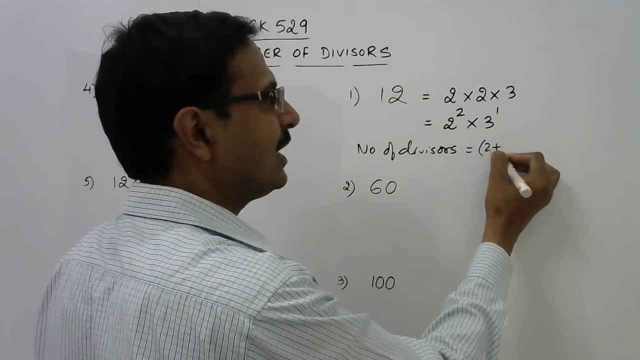 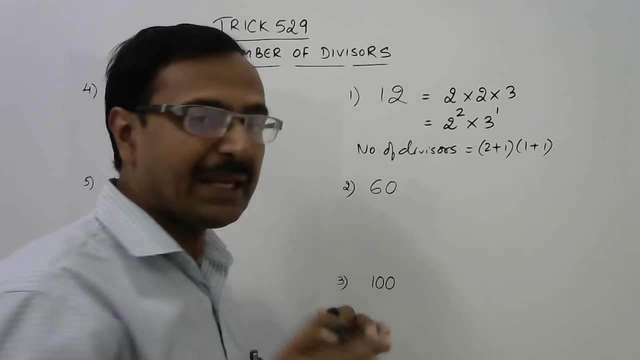 here is 2, increase that by 1.. So 2 plus 1 and the power here is 1.. In the next bracket, increase 1 by 1.. So all the powers are to be increased by 1 and multiplied together. 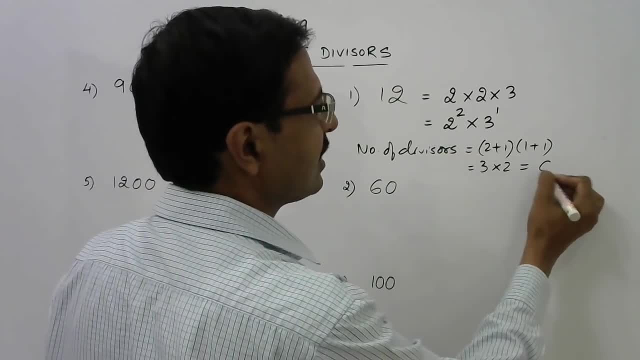 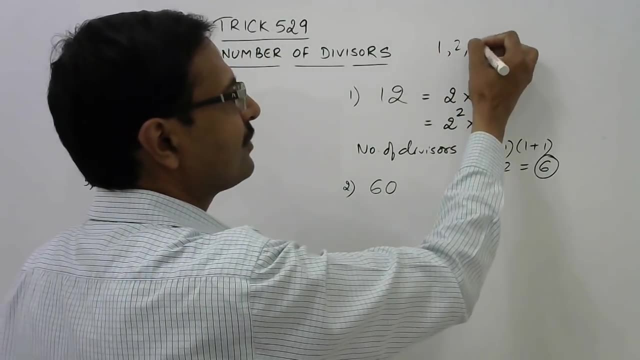 So this is 3 into 2, 6, number of divisors of 12 is 6.. As we can sort out very easily: 1 divides 12,, 2 divides 12,, 3 divides 12,, 4 and 6 and 12.. So these are the 6 divisors. 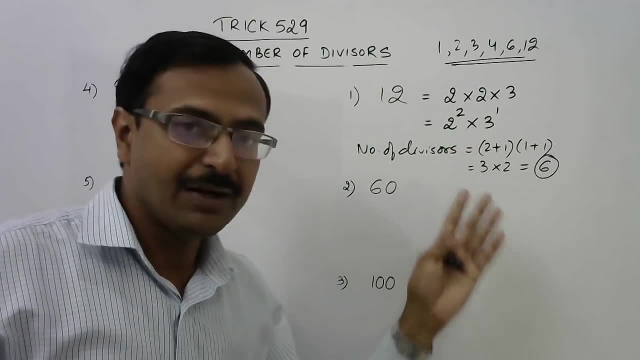 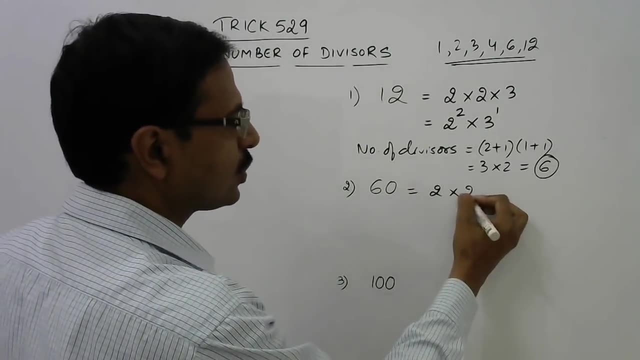 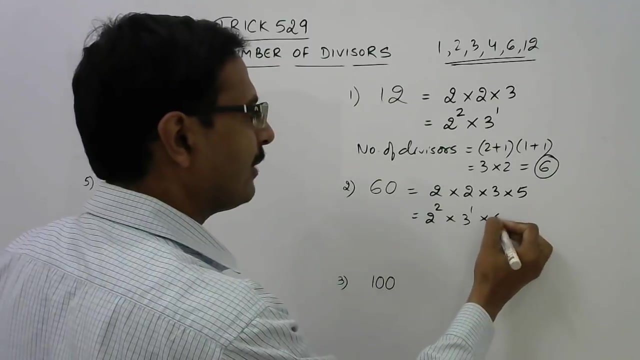 of 12 and the number of divisors can be obtained using this simple method. Let's see 60.. 60 can be written as 2, 30, so 2, 15,, 3 and 5.. So here we have 2 power 2, 3 power 1 and 5 power 1.. Now there are 3 prime factors. So 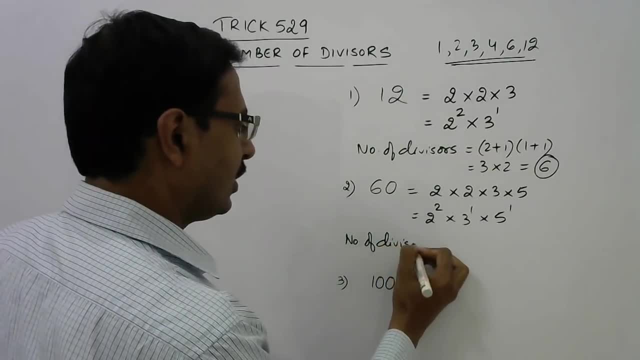 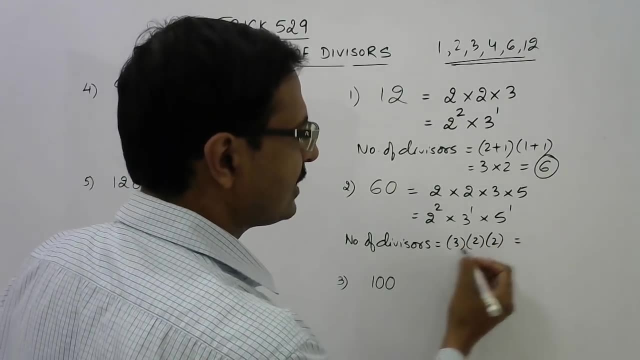 the number of divisors of 60 will be 2 plus 1, 3, 1 plus 1, 2 and 1 plus 1, 2.. Now multiply these 3, 3 to the 6 to the 12. So we have 12 different divisors of 60.. Likewise now. 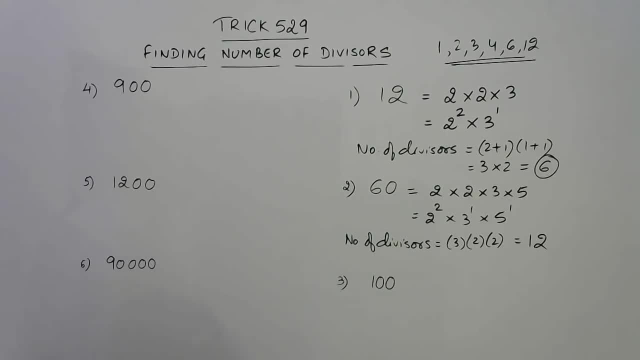 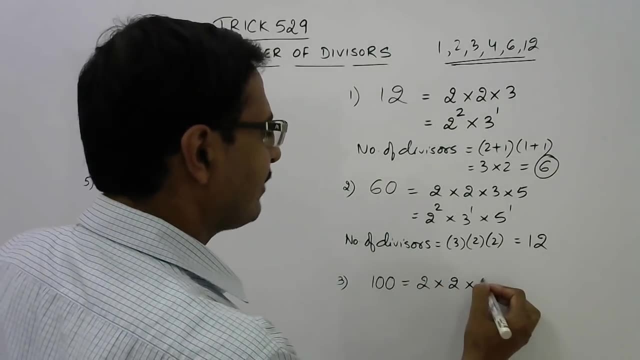 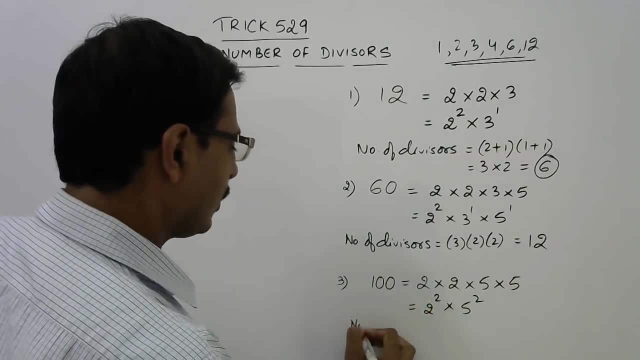 be written as 2 to the 4.. 4 means now 25, so 5 into 5.. So this can be written as 2 square into 5 square And therefore the number of divisors of 100 will be 2 plus 1, 3.. 2 plus. 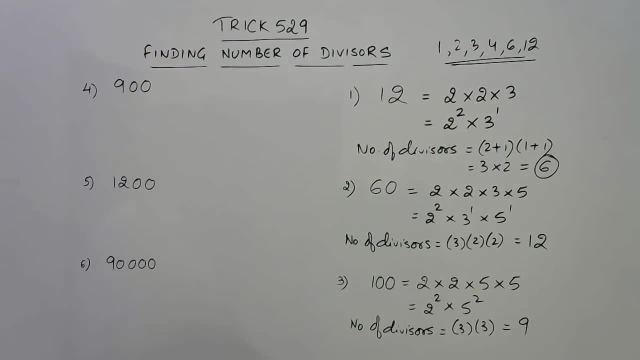 1, 3.. That is 9 divisors. Now take 900.. 900 can be written as 2, 450.. 2, so 2, 25.. 3, 50, 2.. so 45, again 3, 15, again 3 and 5. so these are the factors, prime factors. so this can be written as: 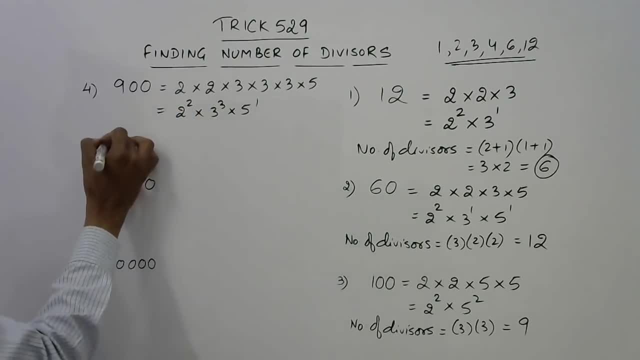 2 square 3 power 3 and 5 power 1, so the number of divisors of the number 900 will be 2 plus 1, 3, 3 plus 1, 4 and 1 plus 1, 2. now multiply them: 4, 3's are 12, 2's are 24, so there are 24 different. 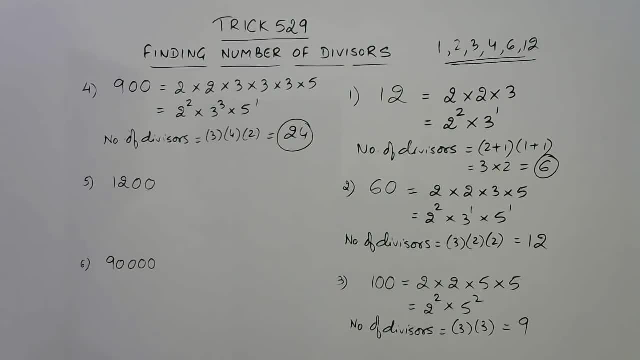 divisors of 900, starting from 1 and ending at 900 each other. now we can make factors of 1200, say 2, 600, 2, 300, 2, 150, 2, 75, 3, 25, so 5 and 5. now write them in the power form. 2, power 4. 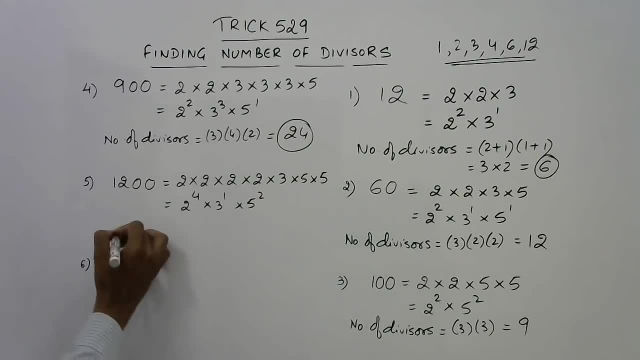 3 power 1, 5 power 2. so the number of divisors of 12 will be 4 plus 1, 5, 1 plus 1, 2, 2 plus 1, 3. so 5, 2's are 10, 3's are 30, so there are 30 divisors of. 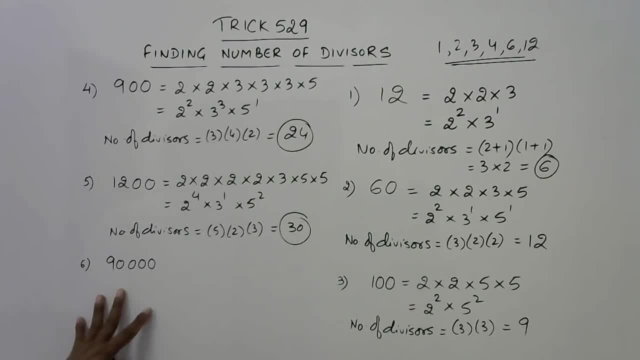 1200. finally, let's take a large example. say this is 90 000, so 90 000. first i'll write it as 3 into 3, 9 and then 10, 4 times. but we cannot make composite factor. 10 is a composite number, so 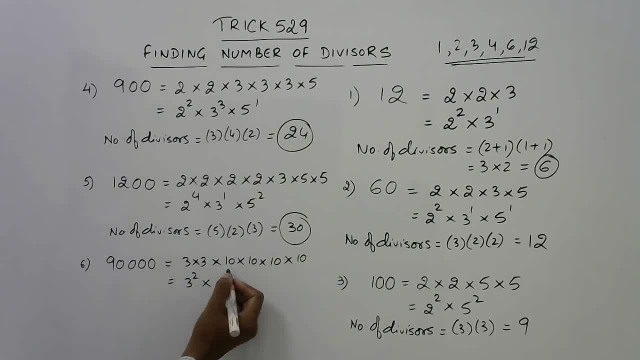 we need to break it down. so this is 3 square. obviously we know that two into five, so we will have four twos and four fives. so now we can find a number of divisors of 90,000, so 2 plus 1, 3, 4 plus 1, 5 and 4 plus 1, 5, so 5 into 5. 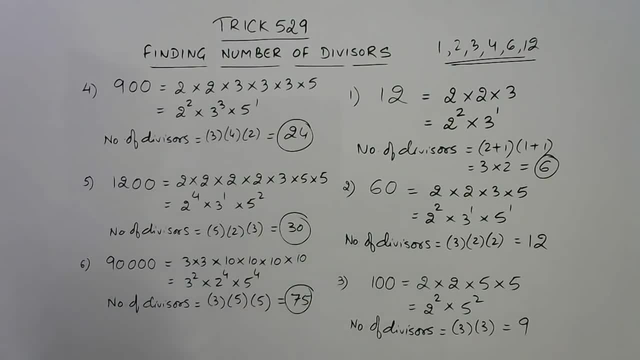 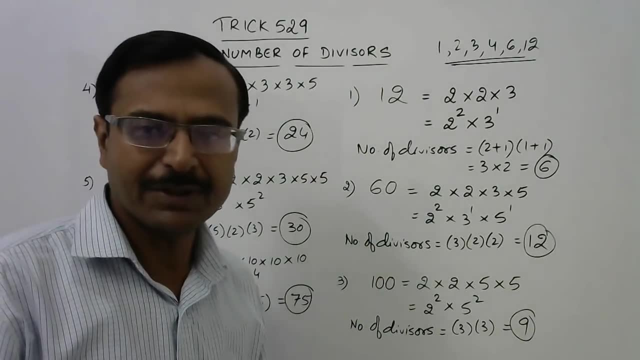 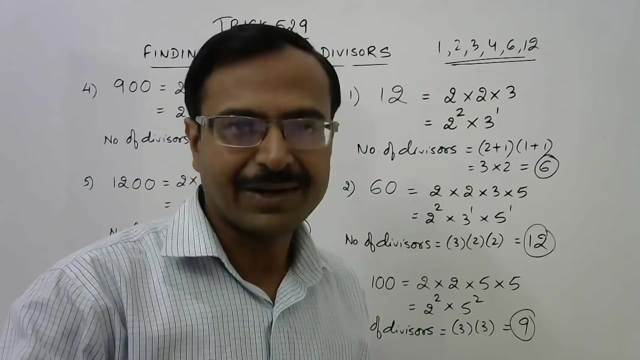 25 into 3, 75, so there are 75 different divisors of the number 90,000. so, friends, you see a simple method and you will be able to find out the total number of divisors of any number. yes, you need to know the prime factorization of numbers. 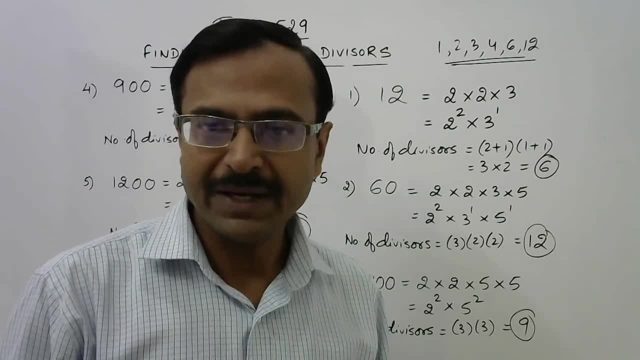 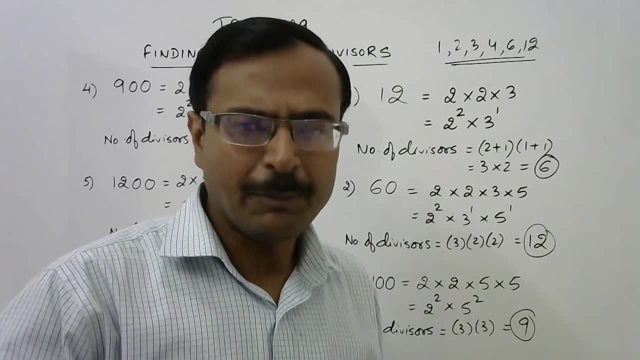 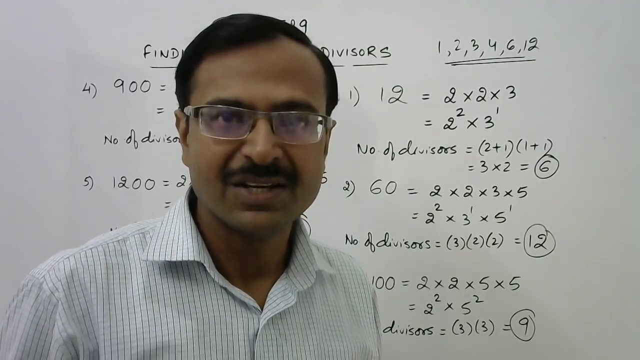 and carry it out very, very quickly. if you spend time in finding the prime factors then obviously this method is going to consume time. so very important method for competitions. these kind of questions, you know they are very frequently asked in all numerical ability tests. so practice them and I am. 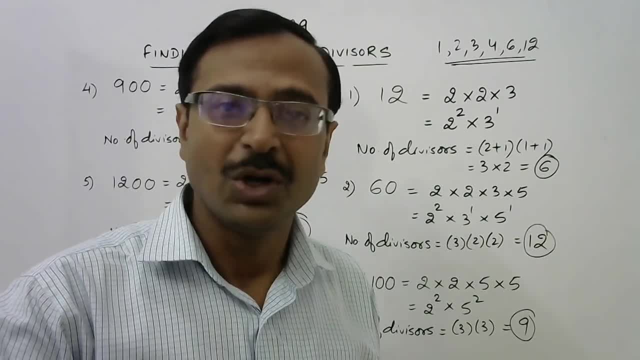 sure you will save a lot of time in competitions. so if you like the video, do share it and subscribe the channel you.